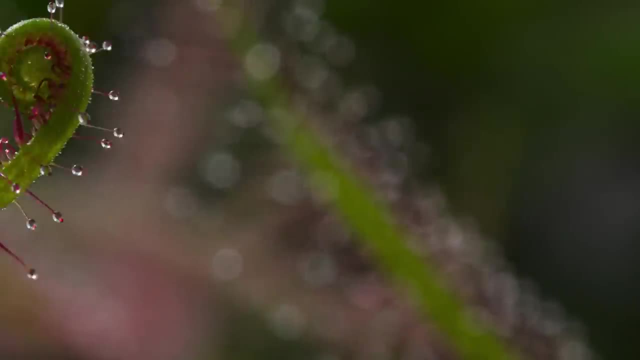 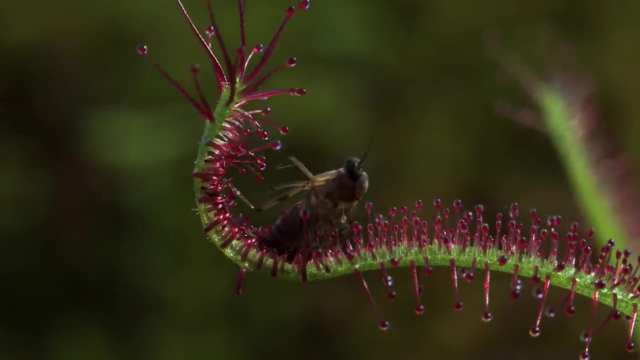 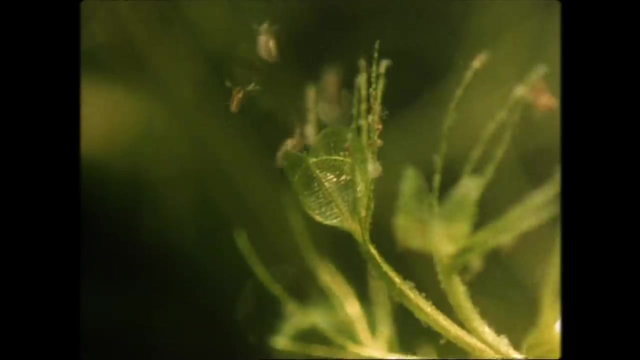 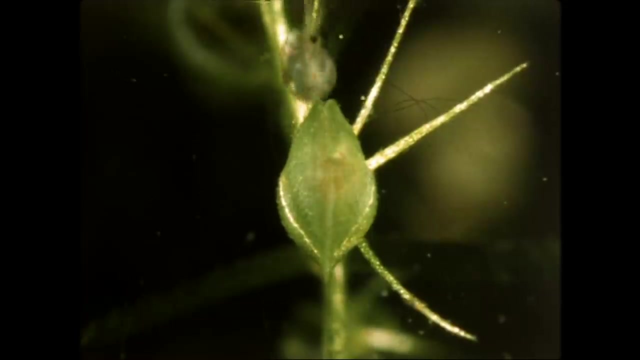 carnivorous plants known to science. Darwin's beloved sundew plant is in the adhesive trap category. This is the most common type of sundew plant which is found in the wild. He knows nothing but the most popular of different plants which get stuck to extremely sticky droplets. 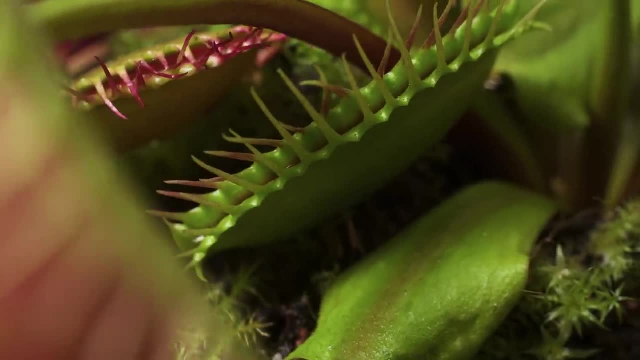 Then there are the pitfall traps, like pitcher plants, where prey falls into the base and is digested. And then there's the suction traps, like the waterwheel plant, where aquatic prey animals get sucked into a one-way trap door. But the most iconic of all carnivorous plants are the snap traps. like the voracious and enigmatic Venus flytrap, Unsuspecting prey, lured by the flytrap's sword, can easily be caught by its own antlers. In the first place, the sundew plant is an animal that is able to move itself into its own body, and its own body can be easily caught by its own body. 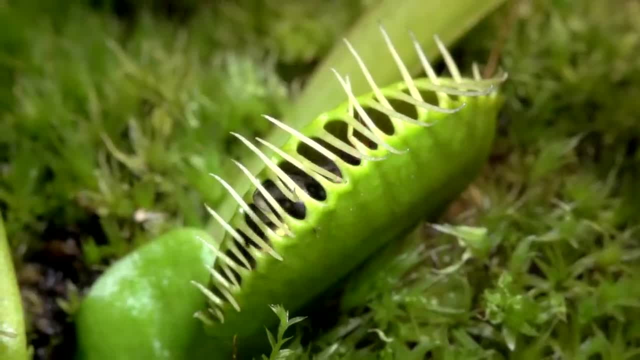 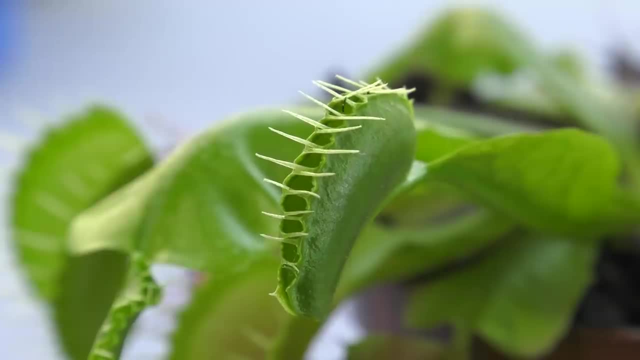 It can also be eaten by its own body, and its own body can be released into its own body. the flytrap's sweet-smelling nectar land in the jaws of the flytrap and quickly find themselves locked behind the teeth of the hungry plant, where they are then digested. 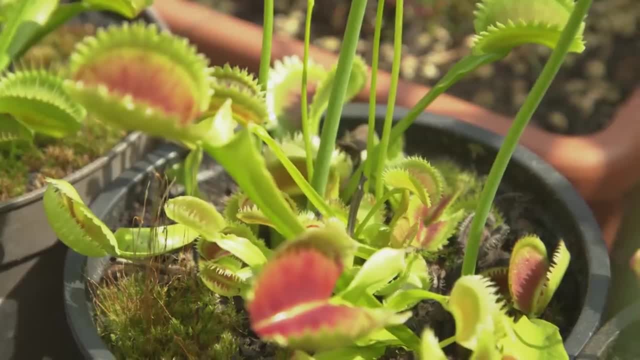 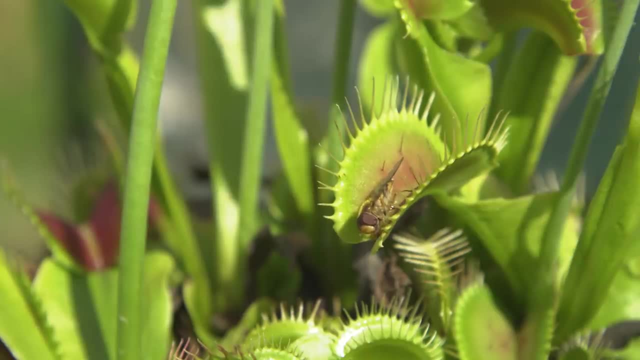 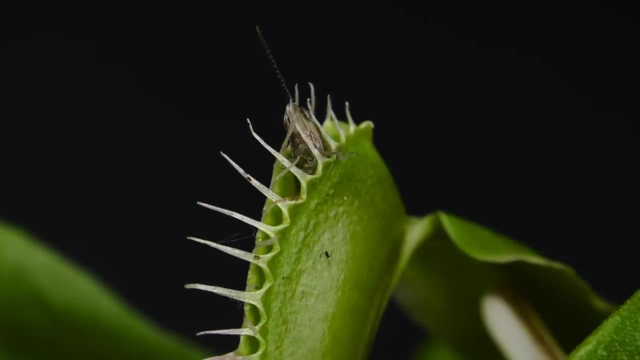 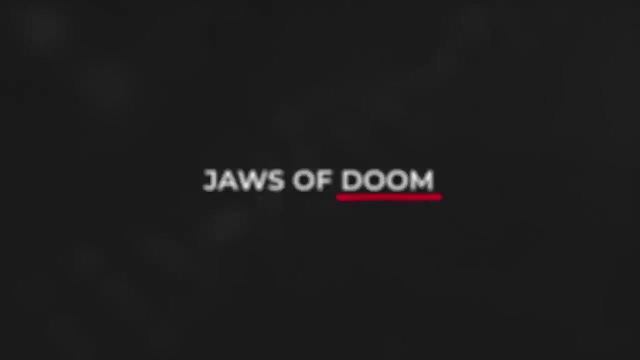 slowly over the course of a week. The discovery of these meat-eating plants changed the very idea of what it means to be a carnivore. But how and why would plants evolve such a taste for flesh? How is it possible for a leafy green to become a deadly predator? 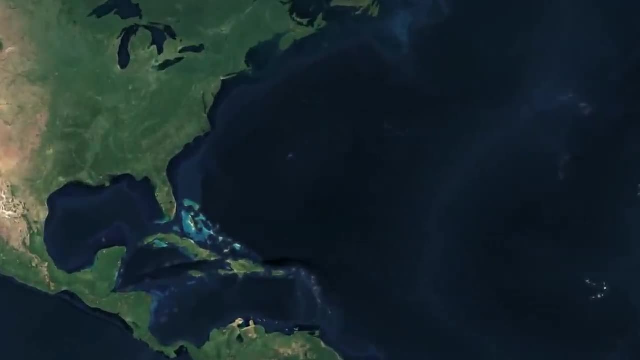 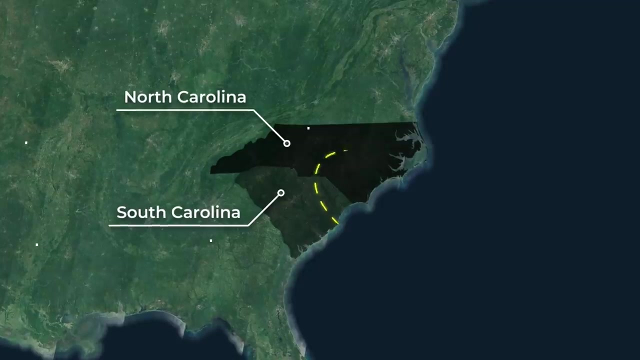 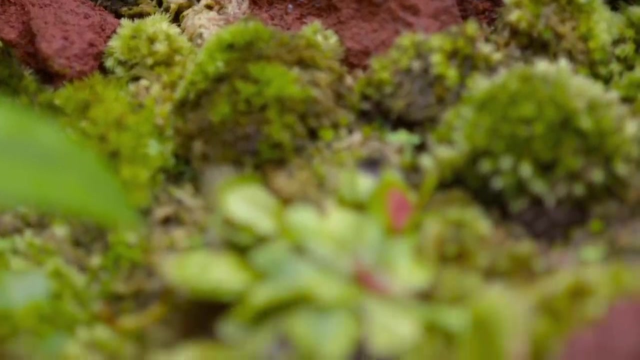 Venus flytraps are naturally found in only one area in the world: in the coastal plains of North and South Carolina, specifically in one small region 200 kilometers across. They are small plants that live in the open understory of their habitat- an understory. 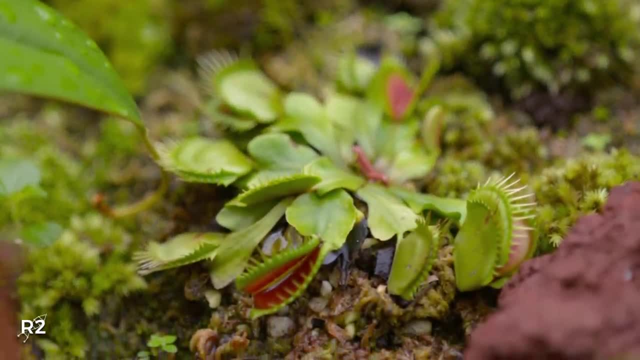 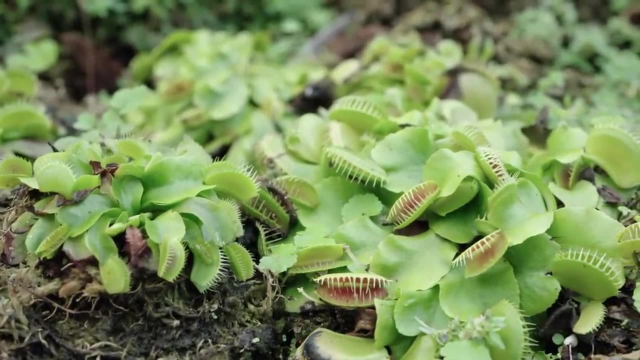 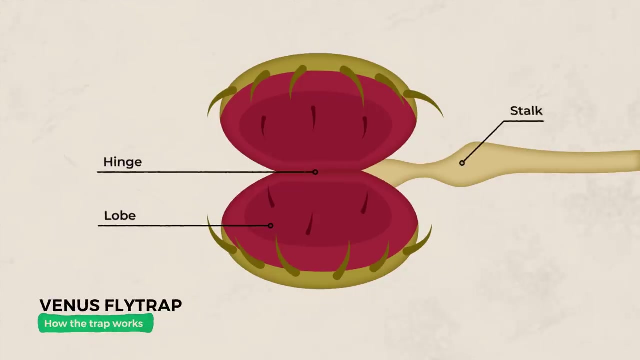 that remains open due to natural fires that burn away the larger shading plants, And down here amongst the marshy grass is where their killing commences. The trap of the Venus flytrap is a leaf with two lobes connected at a hinge on its stalk. 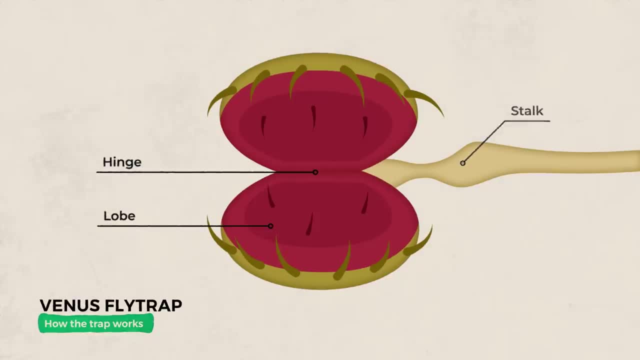 The lobes sit waiting curved in the open position, luring prey insects with sweet-smelling nectar. If something like a fly, spider or beetle lands on or crawls across the gaping jaws, it risks touching any of the flytrap's six sensory hairs. 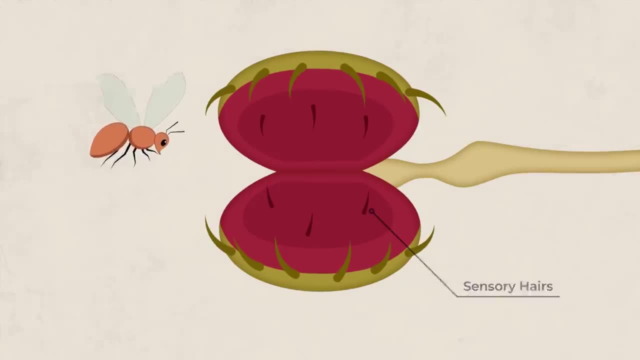 The hairs that give the plant the signal to snap shut. If it touches a single hair, the plant won't budge and the insect is safe for now, But a deadly timer has begun within the plant: a crucial 30 seconds that will determine if 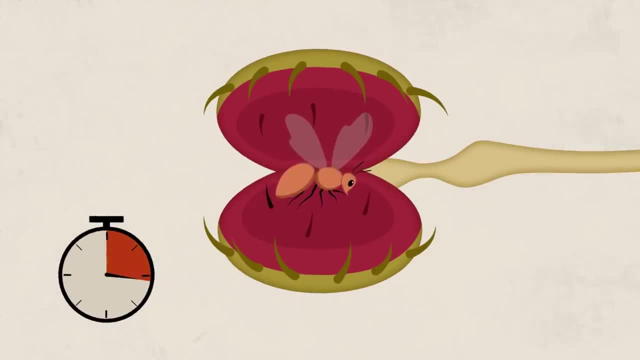 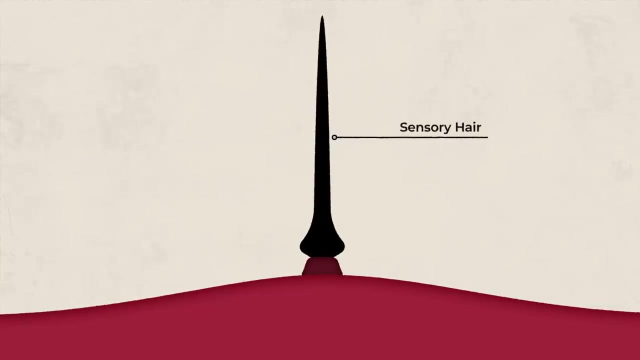 the insect lives or dies. If the insect touches another sensory hair within the 30 second window, the insect is doomed. Upon the second touch, the lobes snap shut faster than the blink of an eye. The plant's movement is controlled by an electrical signal created by the hairs. 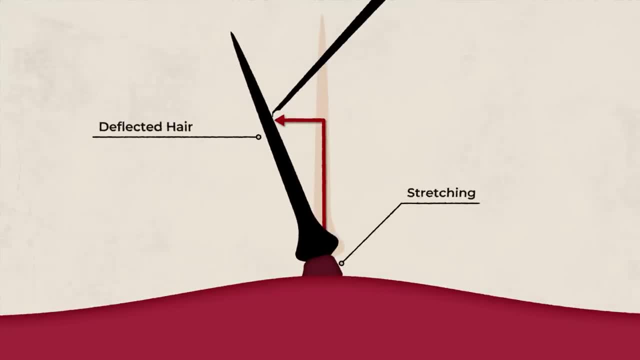 When a hair is bent by touch, it acts as a lever that stretches the envelopes of cell membranes at its base. The stretching causes ion channels to burst open. Positively charged calcium ions flood out, creating an action potential, aka an electrical signal that spreads from the hair over the entire plant. 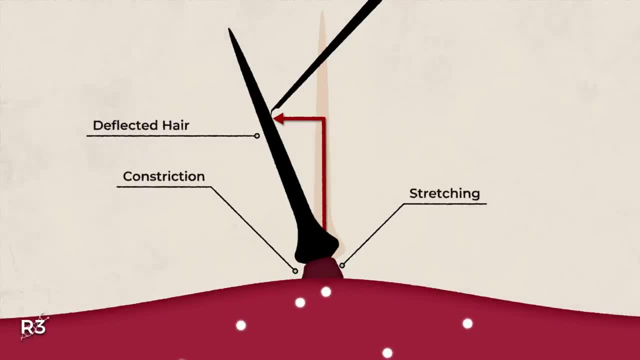 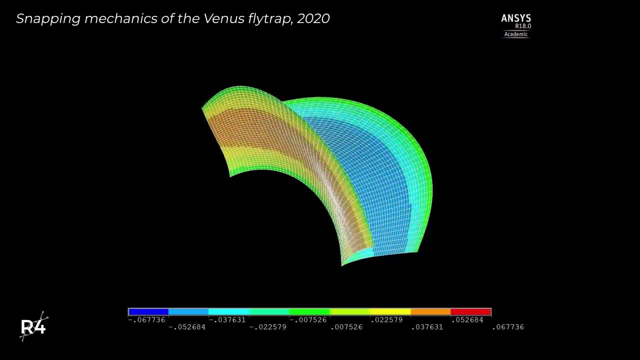 If the plant is bent by touch, the lobes snap shut faster than the blink of an eye. After two action potentials, the trap snaps shut. The initially concave trap lobes move towards each other and eventually change to a convex state. 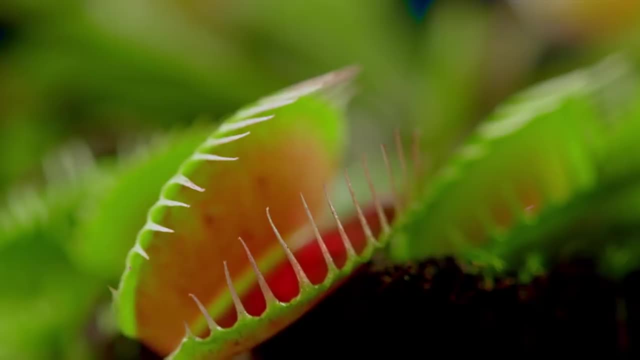 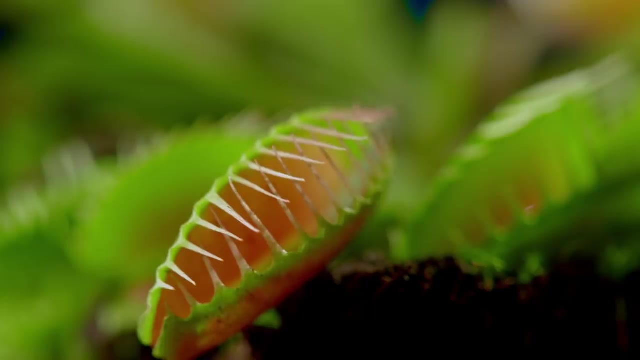 The reason it needs two triggers within a 30 second window is to prevent the plant from closing erroneously and wasting energy for something like a raindrop or a twig. But how does a plant know when 30 seconds have passed? How does a plant tell time? 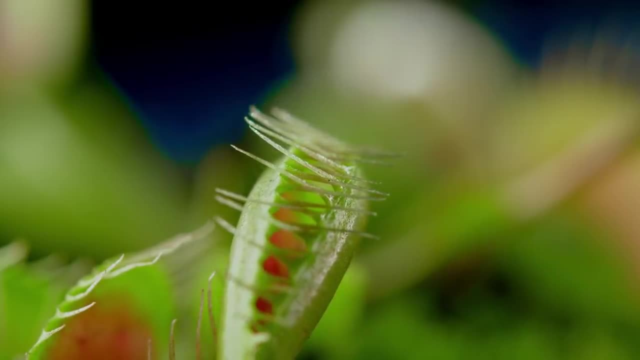 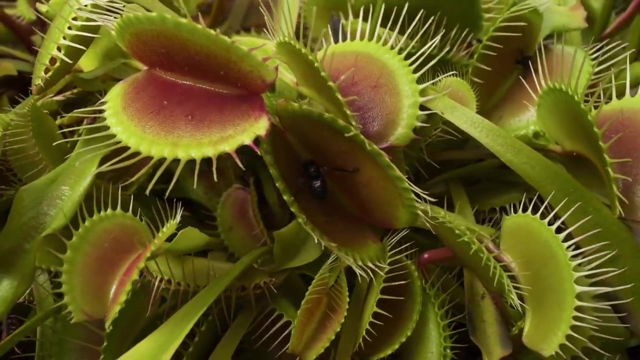 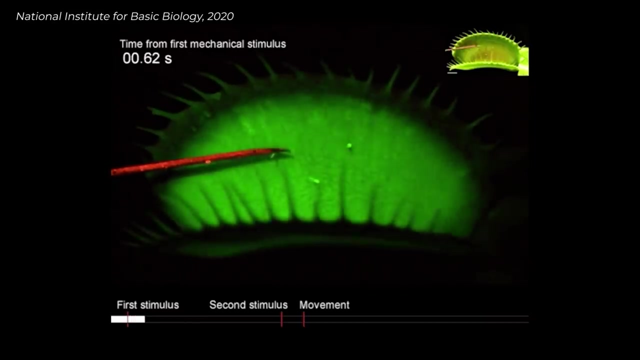 Researchers had a hunch that it had to do with the changes in calcium concentrations inside the leaves. To test this, they genetically modified Venus flytraps to emit green fluorescence when calcium ions were present in the leaf cells. When the first hair is touched, a flood of green overtakes the leaf, showing a big presence. 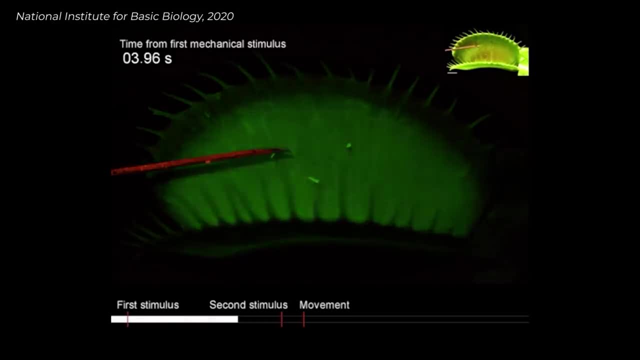 of calcium ions, But as the seconds pass, the concentration slowly starts to drop. But if a second hair is touched, the calcium concentration is reduced. The first hair is touched, the calcium concentration is reduced, But if a second hair is touched, the calcium concentration is reduced. 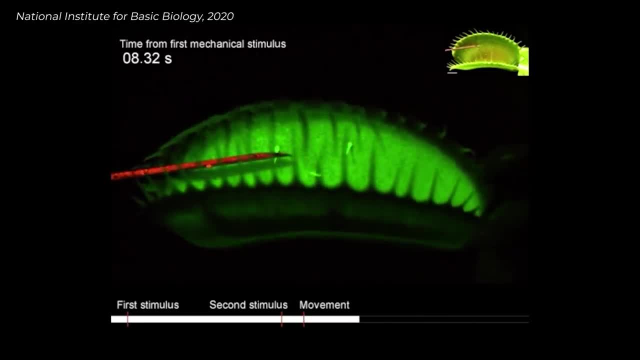 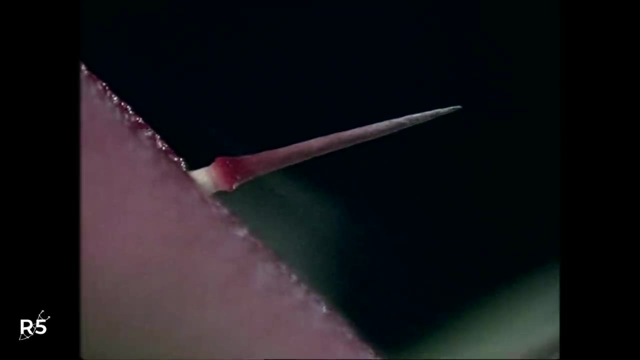 The calcium concentration again increases, flooding the leaf with even more green. It's only when a certain threshold is reached in the calcium concentration that the trap snaps shut. This threshold can only be reached if the two stimuli occur within 30 seconds. But the timed triggers are not the only way. a Venus flytrap ensures it eats only the things 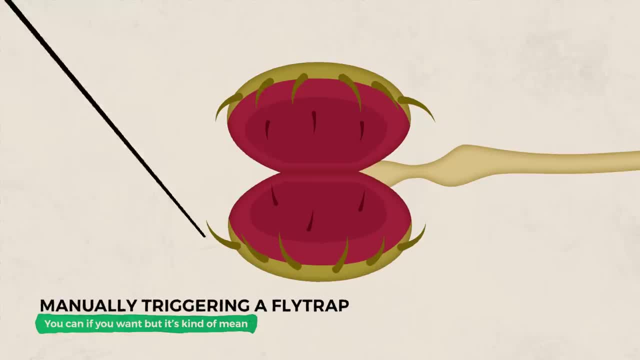 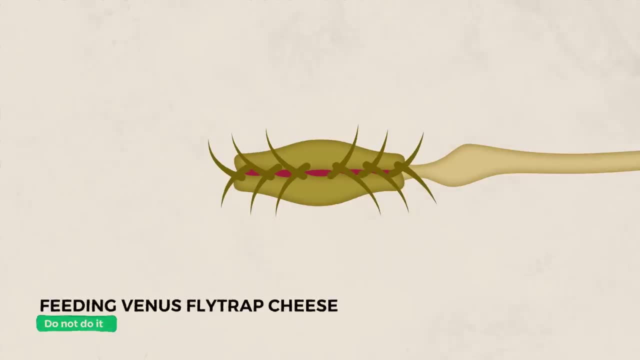 it wants. If you happen to have a pet Venus flytrap, you may realize you can trigger two different hairs yourself, causing it to snap shut. This may tempt you to feed it cheese, like Darwin did with his sundew plants, But if you did, you'd end up disappointed. 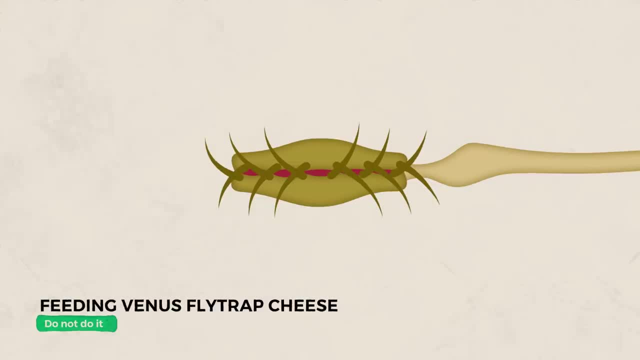 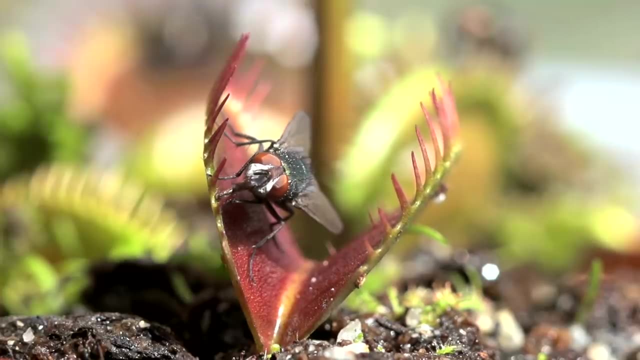 You could indeed get the flytrap to close on the cheese initially, but after a few hours it will reopen, rejecting your generous gift. That's because the plant requires sustained wiggling within its jaws to fully seal and begin the deadly digesting process. 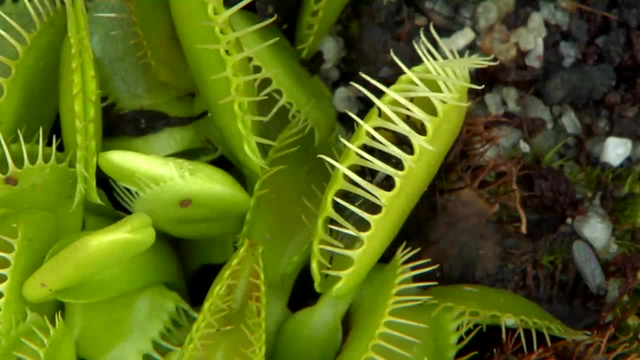 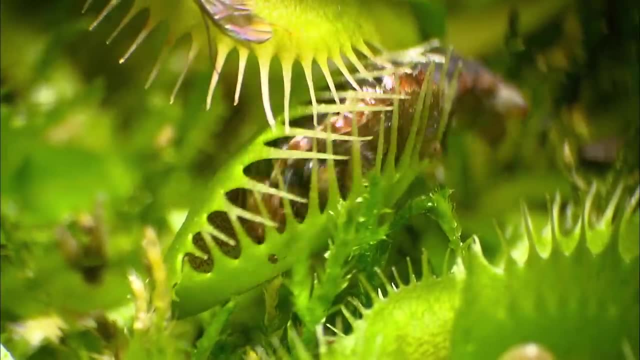 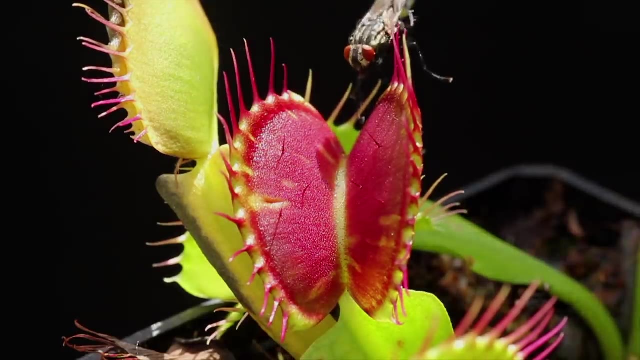 This ensures it's using its digestive resources only on hearty insect meals. But once a wriggling bug does cause the trap to fully seal, it's no longer a mouth but a stomach. Digestive juices flood into the closed trap, The pH drops dramatically and meat-digesting enzymes similar to ones in our stomachs. 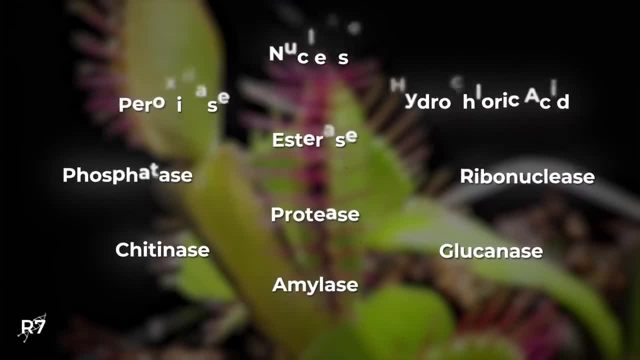 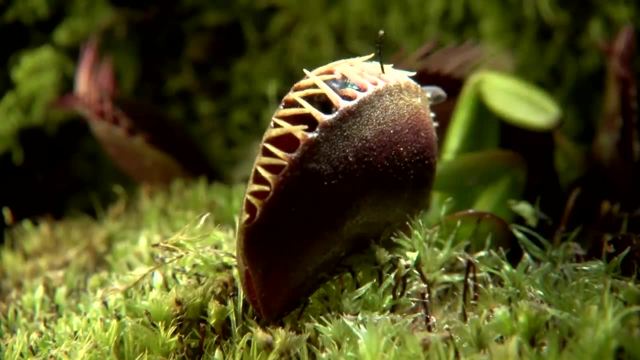 start to break down the trapped creature. The more the prey fights and wriggles, the more digestive enzymes are released. If you're a bug, the more you struggle, the faster you die Slowly. over the course of a week or so, the insect's body is liquefied and the lining 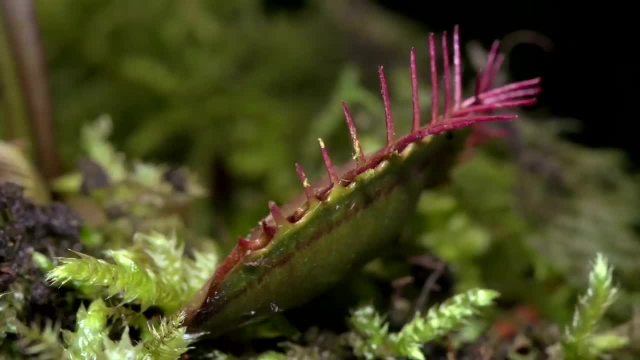 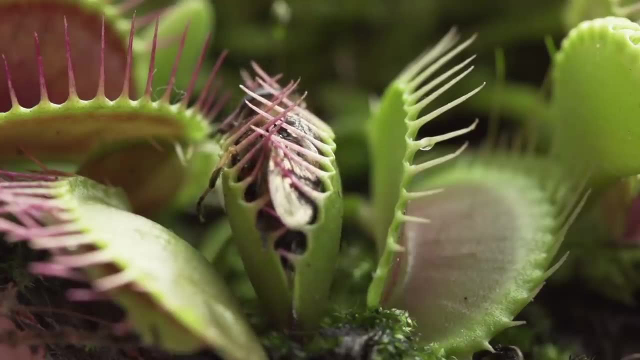 of the trap absorbs the nutrients. It's an impressive, if not a bit unsettling, survival strategy, and it's hard to look at this small plant and understand how it came to be. How do plants make the jump from getting all their nutrients from the soil and the sun? 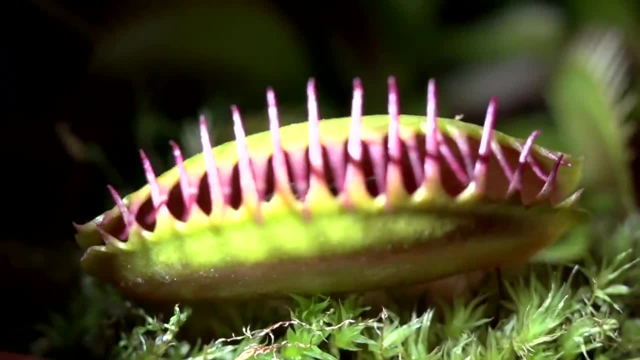 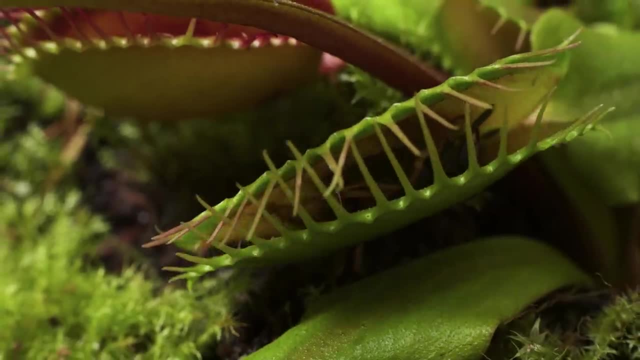 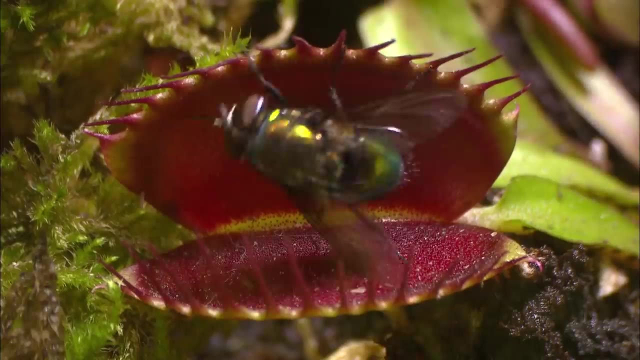 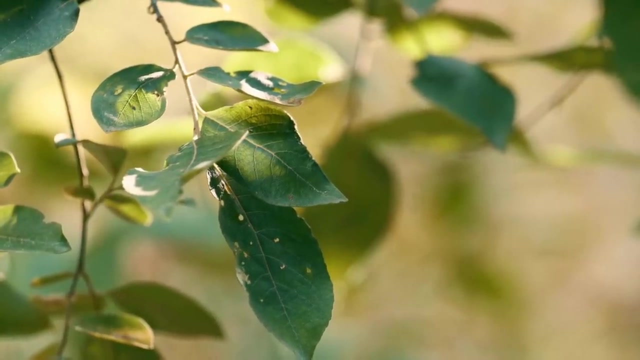 to luring it into the trap. Well, the Venus flytrap does extract some energy from its food, like we do. What it's really after when it kills prey is not the insect's calorie content, but rather its nitrogen. Plants need nitrogen in order to successfully carry out photosynthesis, as it's a major 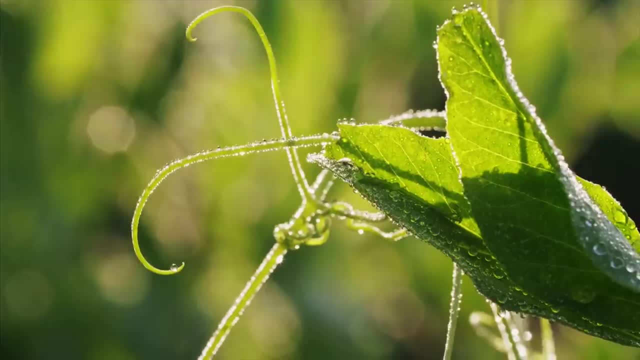 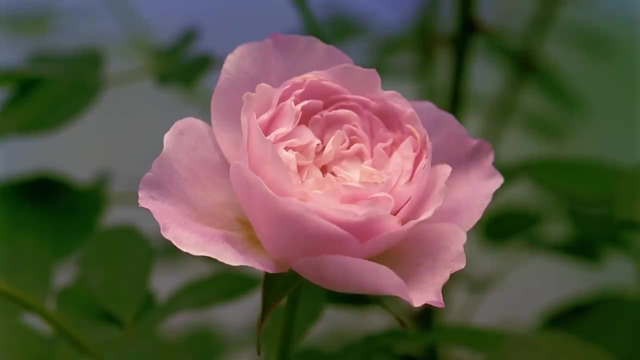 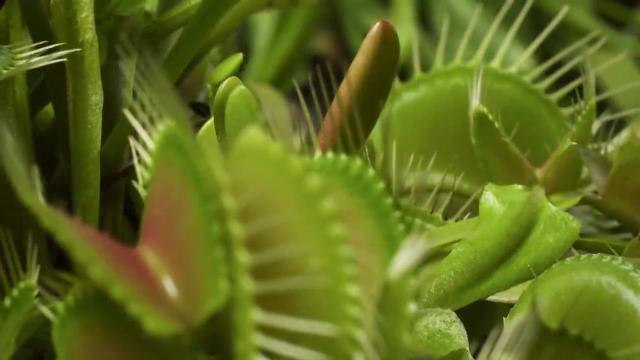 component of chlorophyll. It's also a major component of amino acids, The building block of proteins, and is needed for general growth and regeneration in the plant. Without nitrogen, a plant will wither and die, And this could be a major problem for plants growing where the Venus flytrap does. 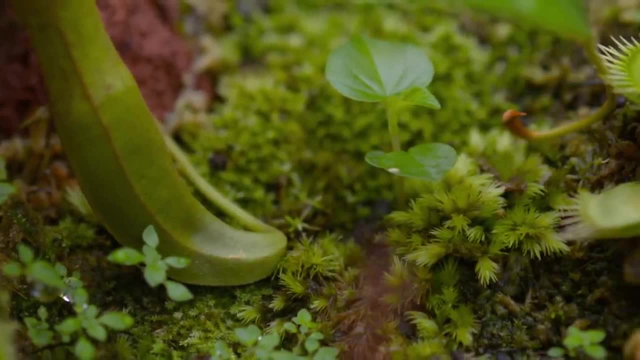 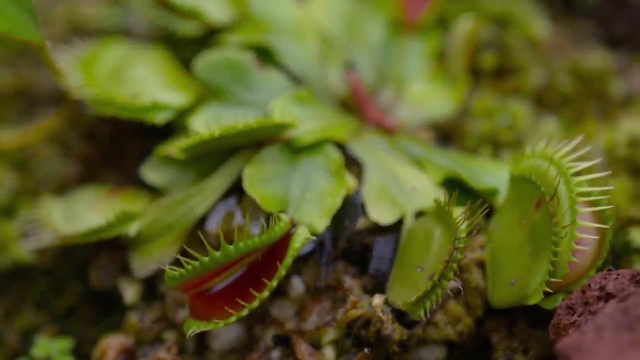 That particular area of the Carolinas where they live has soil that is extremely acidic and nitrogen deficient, But this lack of nutrients is no problem for the Venus flytrap, which gets between 50 and 75% of its nitrogen from chowing down on insects. 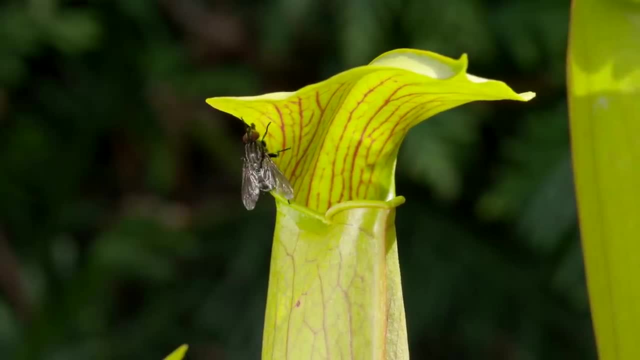 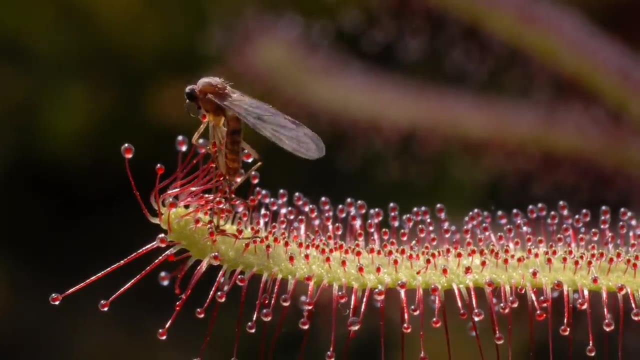 A similar story is true for the other carnivorous plants. Pitcher plants, for example, grow in marshy, nutrient-poor soil, as does the sundew. It seems pretty clear, then, that carnivory evolved in plants to cope with nutrient-scarce. 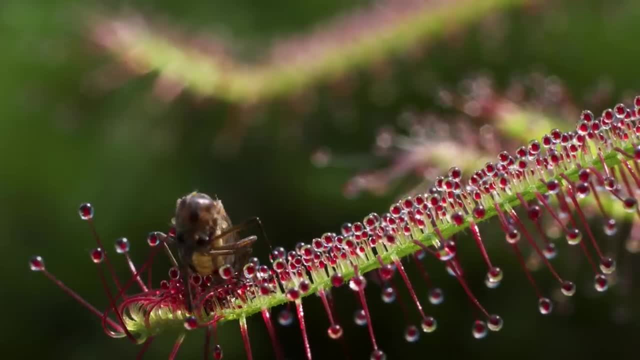 soils. That explains the why, But how does a plant evolve from a purely photosynthetic life to a meat-eating one? To get to the bottom of this story, I'm going to talk about the Venus flytrap. The Venus flytrap is one of the few plants in the world that can survive in the sun. 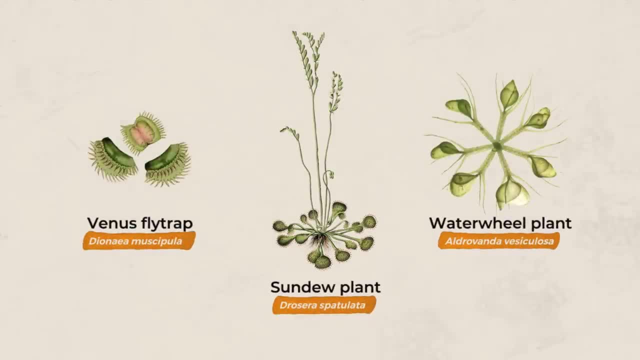 To get to the bottom of this question, scientists examined the genomes of three related carnivorous plants: The Venus flytrap, the aquatic waterwheel plant and the sundew plant. All of these plants use motion to capture prey and shared a common ancestor about 70. 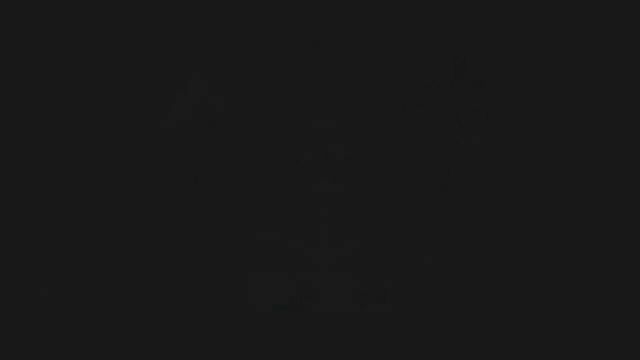 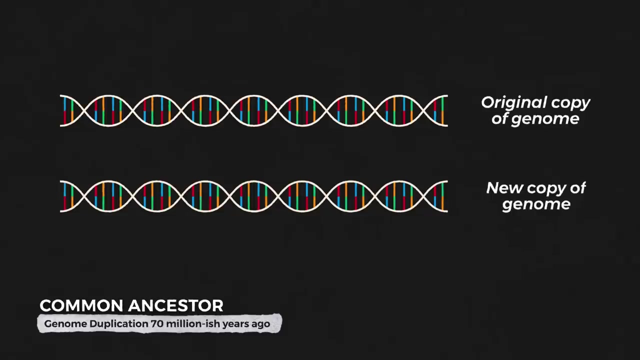 million years ago. Researchers realized that around this time, 70 million years ago, these plants' common ancestor underwent a whole genome duplication, generating a second copy of all of the Venus flytrap's DNA. This duplication enabled the plants to keep one copy of each gene with the original function. 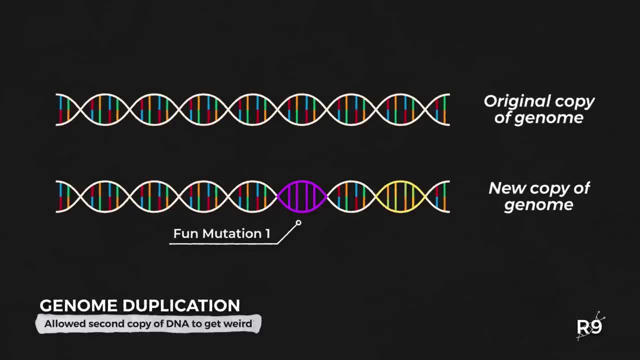 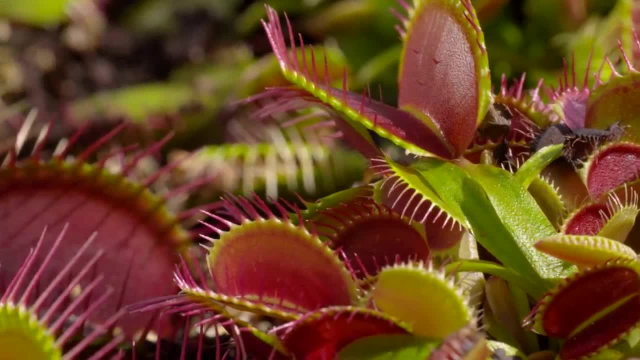 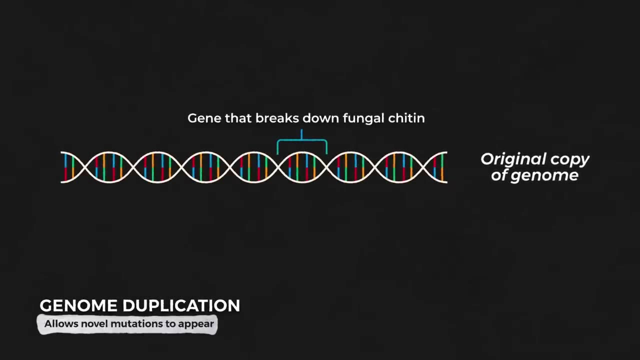 The second copy was thus freed up to be tinkered with where mutations could be tolerated. Eventually, these additional gene copies could start to mutate in a way to fulfill an entirely new role. For example, plants typically produce enzymes that break down a polymer called chitin. as 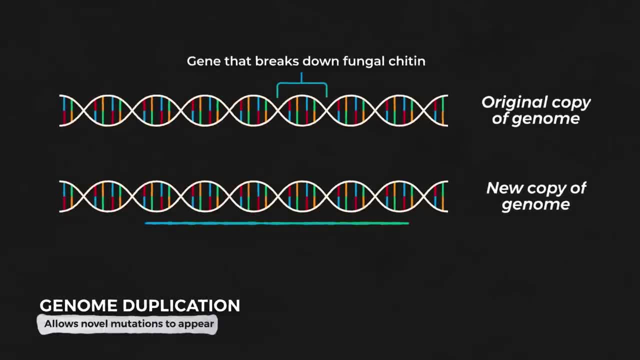 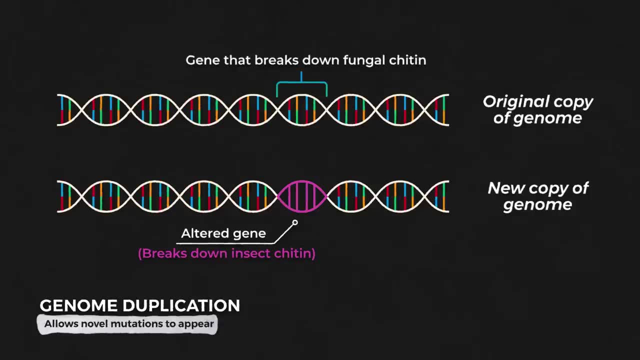 a defense against fungi, But with a duplicated genome. carnivorous plants have repurposed the enzyme to digest insect exoskeletons, which are also made of chitin. Typical plants also use their root system to reach for and absorb nutrients underground. 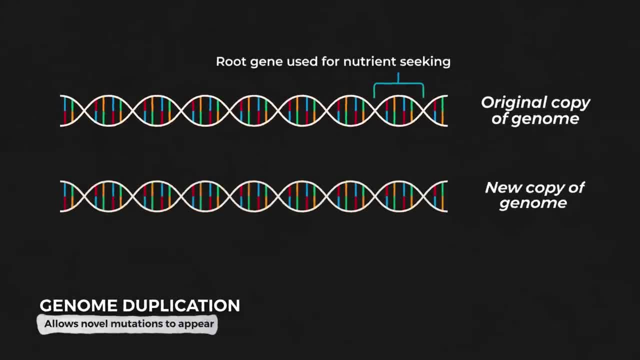 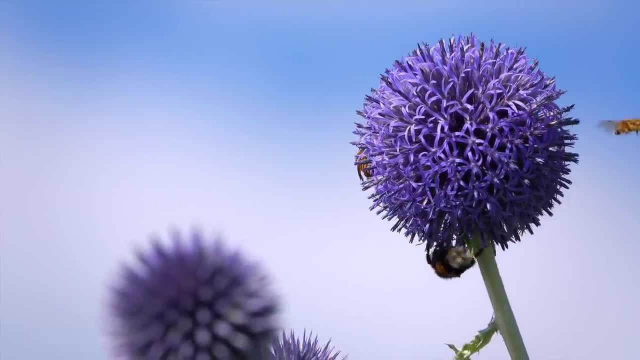 In carnivorous plants, these genes are repurposed for their traps, which are now the primary nutrient absorber. Regular plants also produce sweet nectar to attract pollinators, and now carnivorous plants repurpose these nectar genes to produce new nutrients. 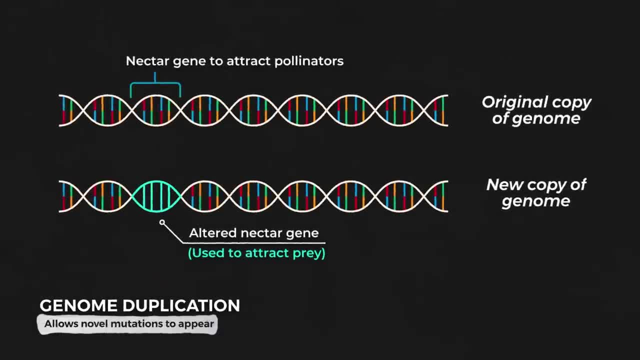 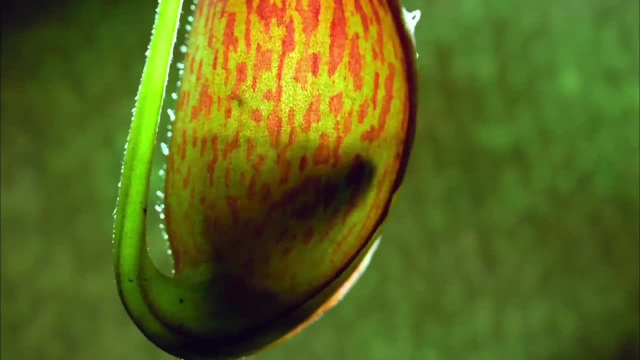 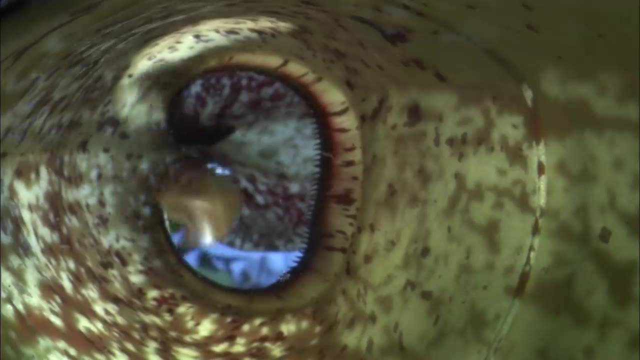 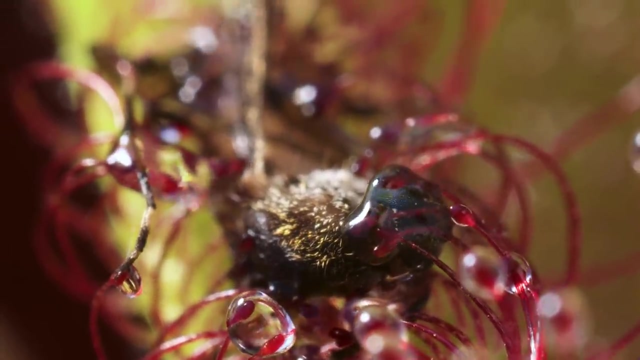 gene families were expanded. Gene families that create digestive enzymes, for example, became upregulated. This allowed plants to fine tune their different carnivorous strategies. Then, once the plants were effectively exploiting their new niche and absorbing nutrients from living prey, their traditional leaves and roots were no longer confines as naturally. 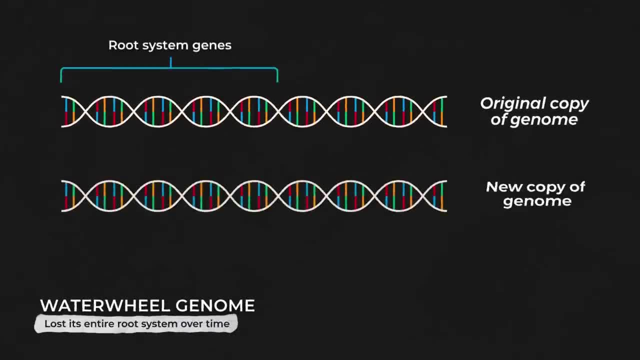 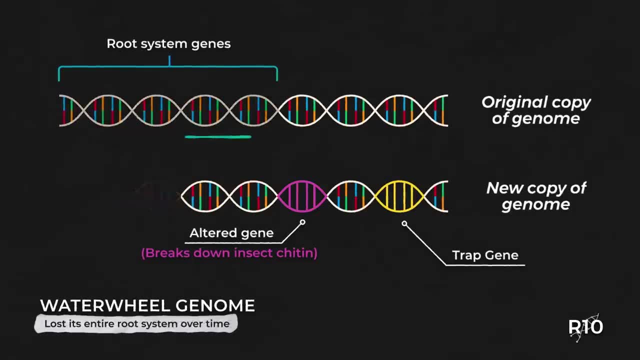 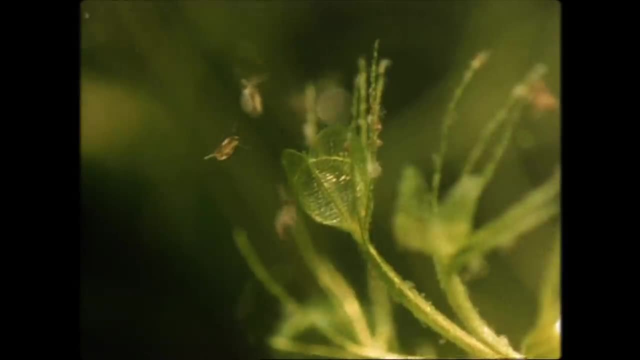 as necessary. many genes that were not involved in carnivorous nutrition began to disappear. For instance, aquatic waterwheel plants eventually lost their root system altogether As a result of losing many of these typical plant genes. the three plants observed in the study are some of the gene-poorest plants to be sequenced to date, meaning they have 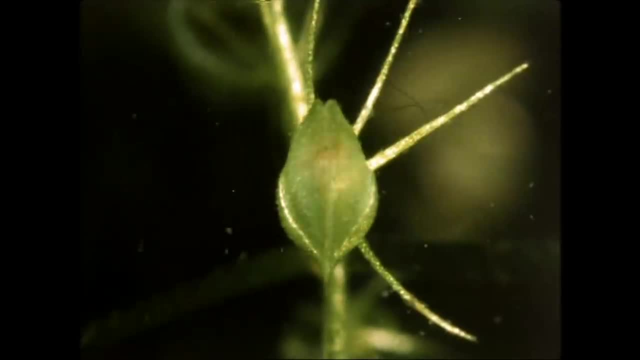 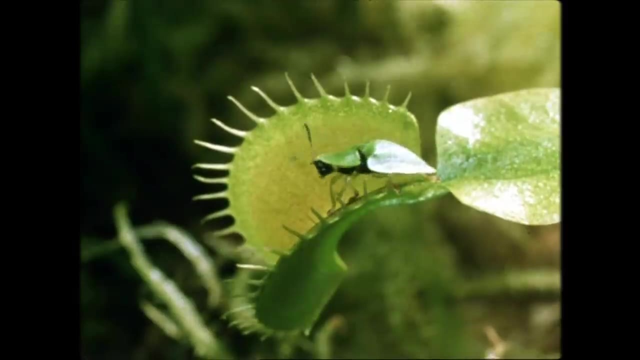 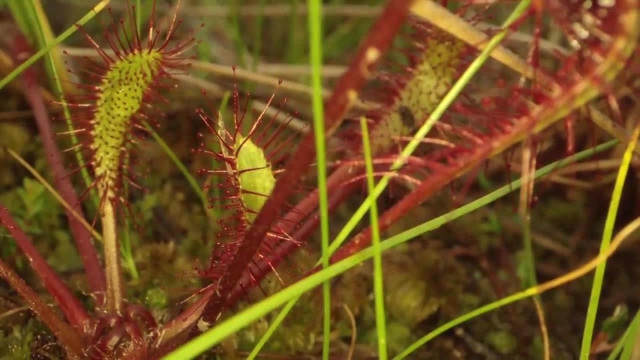 among the smallest genomes ever discovered in plants. All carnivorous plants seem to have followed this genetic roadmap to get to where they are today. However, surprisingly, it was not a genetic event that happened just once in a single common ancestor belonging to all carnivorous plants. 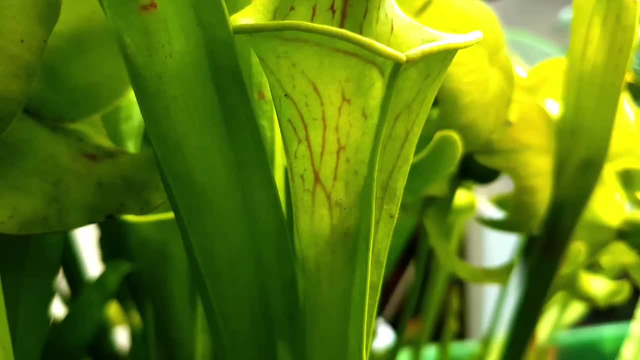 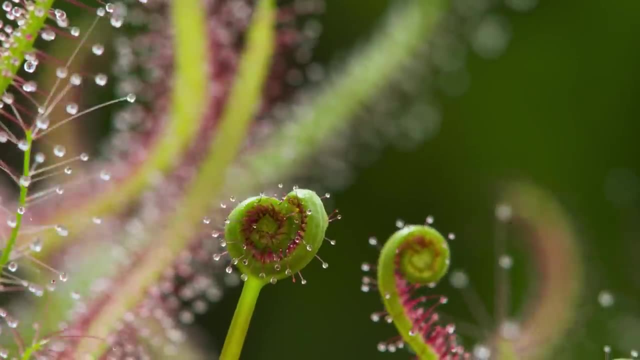 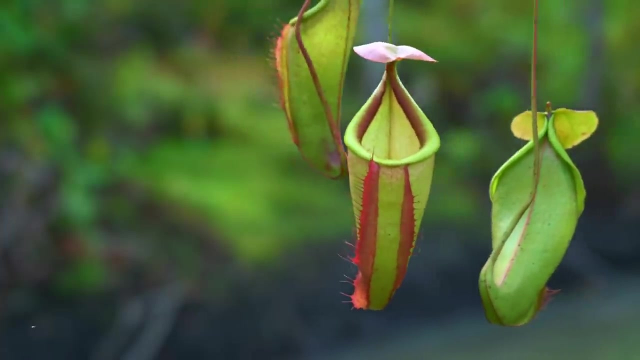 It's a sequence of events that has happened several times completely independently from one another. Carnivory in plants has evolved as many as six separate times. Some carnivorous plants that even look nearly identical turn out to be nowhere close to each other on the evolutionary tree. 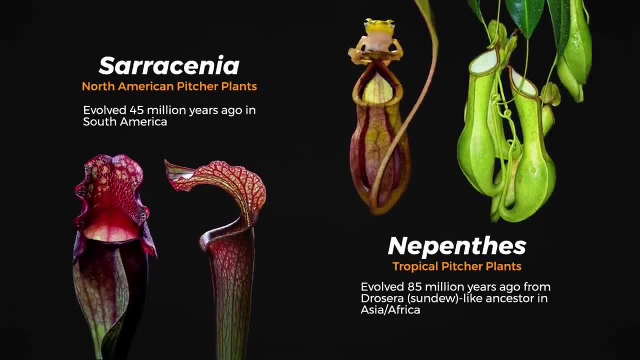 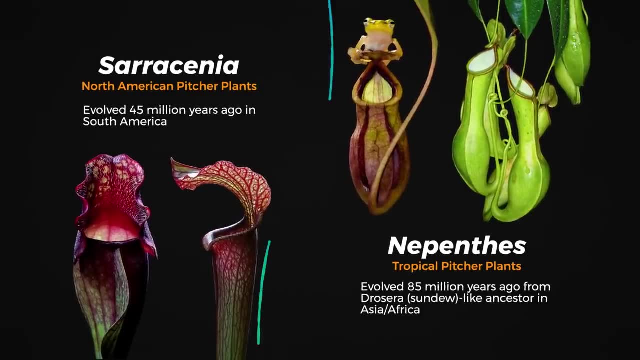 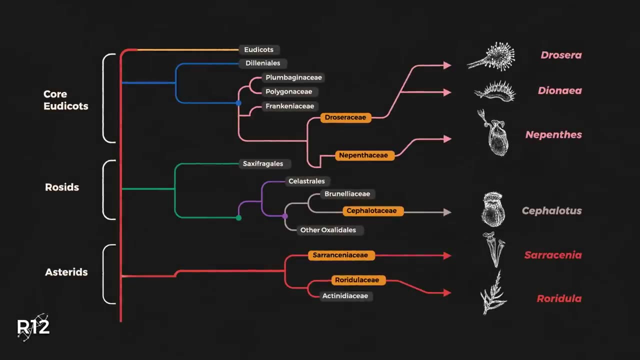 Both families of pitcher plants- the tropical genus and the North American genus- look almost exactly the same and catch prey in the same exact way, with their deep, slippery, pitcher-shaped leaves full of digestive enzymes. Yet they became carnivorous at separate moments in history on different branches of the tree. 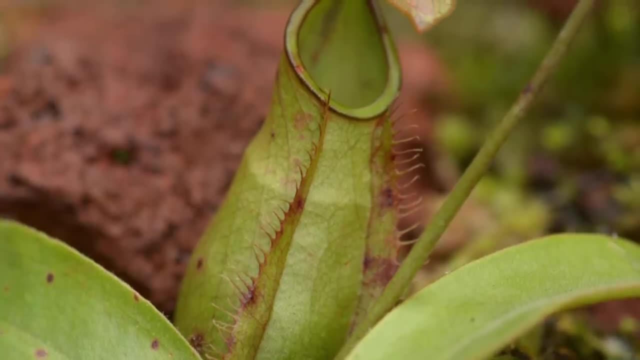 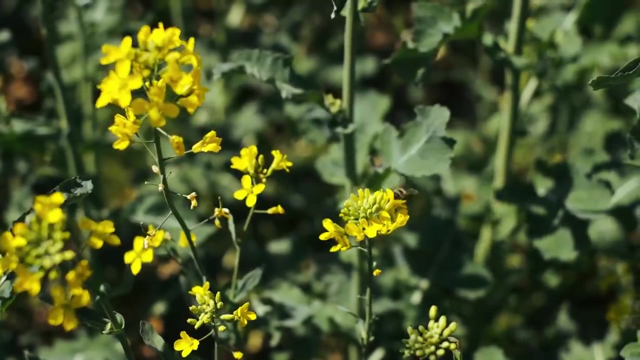 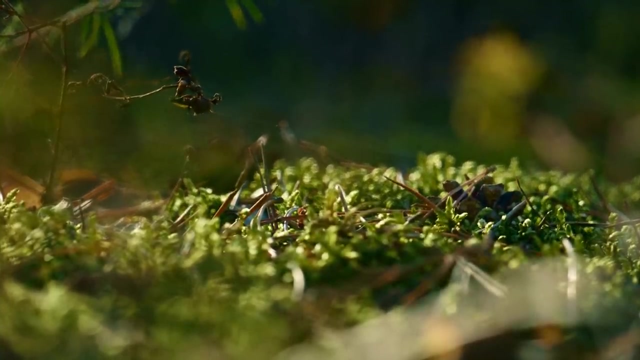 of life. These discoveries reveal something surprising: most plants with leaves and roots contain the material necessary to survive. It is necessary to become carnivorous, meaning the path to carnivory is open to all plants Given the right circumstances, in an environment with little nitrogen and with enough time. 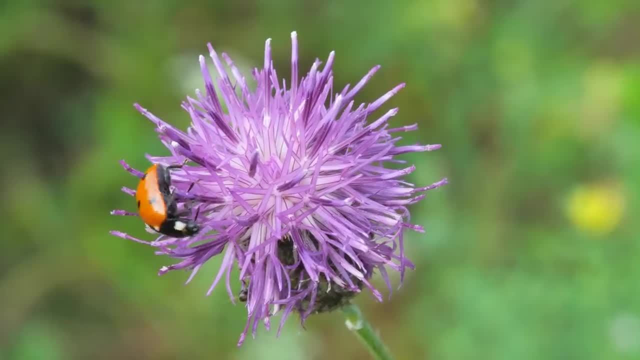 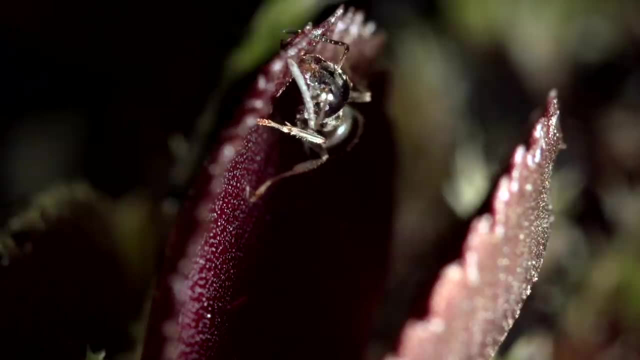 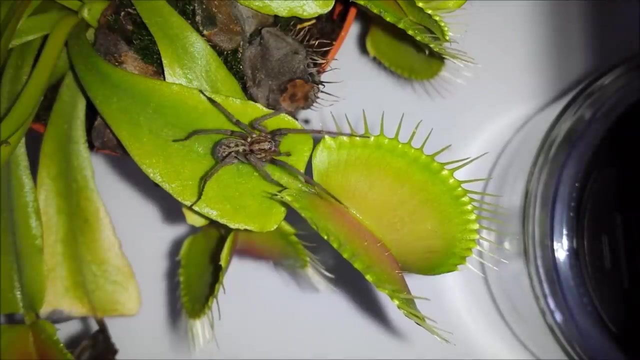 some photosynthetic plants we know today can, and likely will, evolve into brand new types of predatory meat-eating plants. The shapes they take may be similar to the ones that exist now, or new forms may come about altogether. Plants are remarkable at adapting to adverse conditions, and only time will tell which. 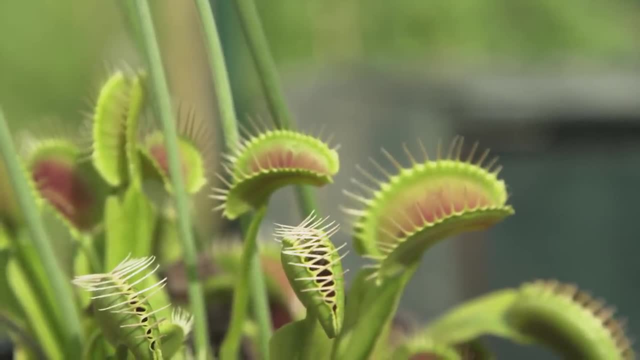 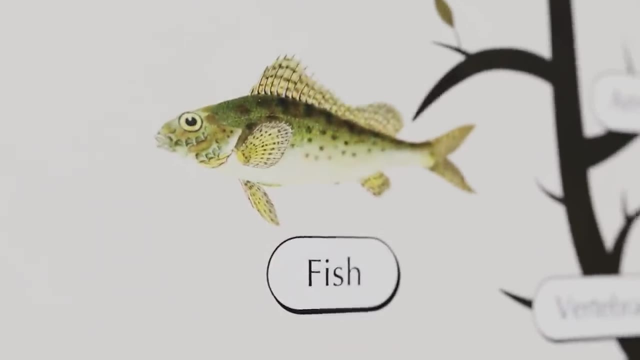 plants will eventually be chowing down on their meaty neighbors. On this channel I talk a lot about genetics and evolution and point to a lot of phylogenetic trees. To me, it's literally the coolest thing ever to get a glimpse back in time to understand. 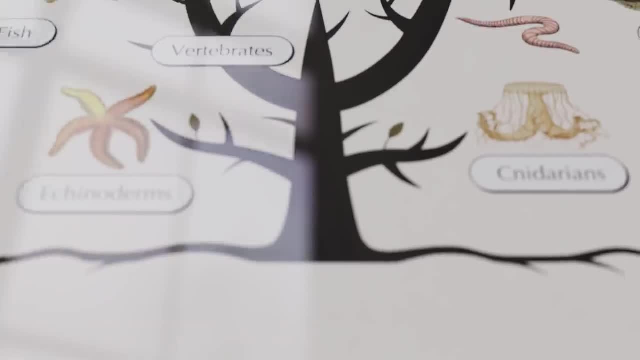 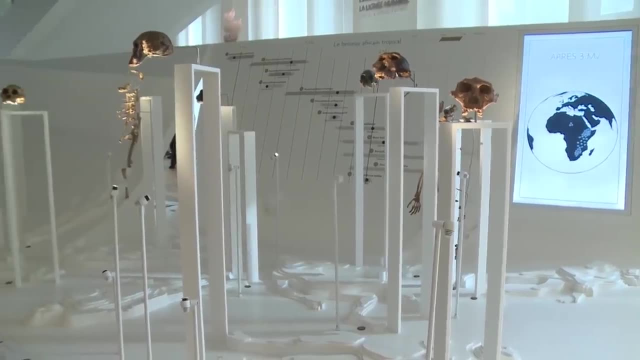 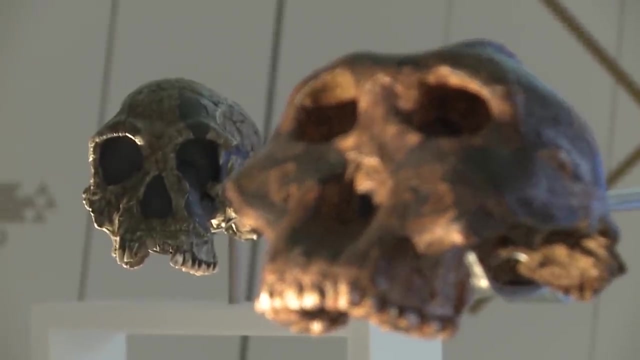 when different organisms diverged on the tree of life, to see the infinitely complex branches spreading and unfolding over time. But it's understandable to ask: how do scientists know that stuff? For years scientists had only comparative anatomy to go on. Darwin, for example, could only look at the beaks of finches to observe their differences. 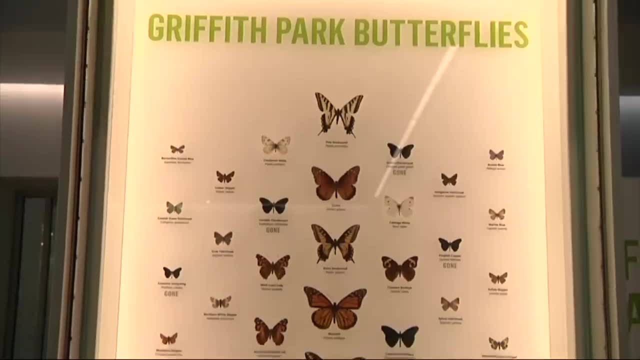 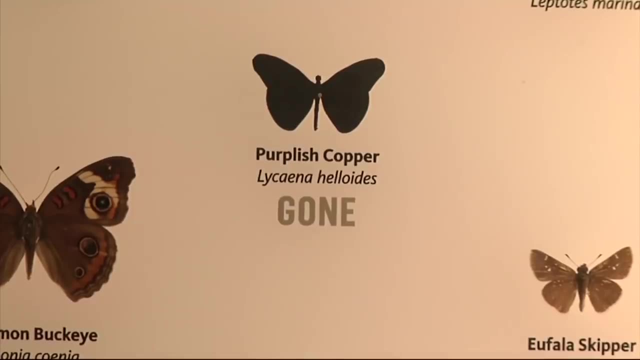 and to attempt to discern the different birds' relatedness, And when comparing two organisms that don't even look the same. comparing anatomy can't tell you that much about their connectedness. So for a long time it was understandable that people looked at the huge array of life. 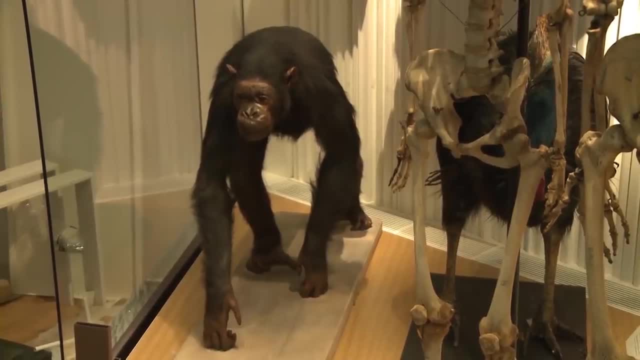 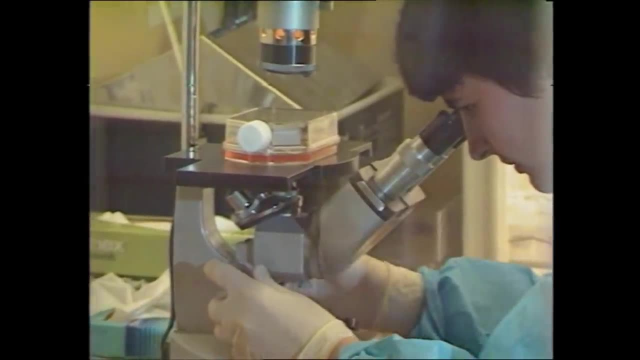 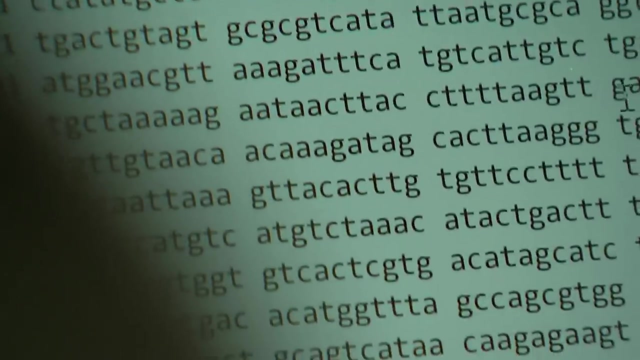 on Earth and refused to believe it was all related, that every living organism on this planet shares a common ancestor. But then came the discovery of DNA. We can now see that all life does look the same at the molecular level, meaning that all life shares a genetic language. 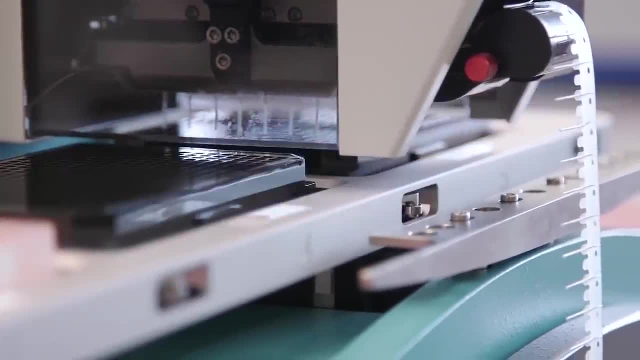 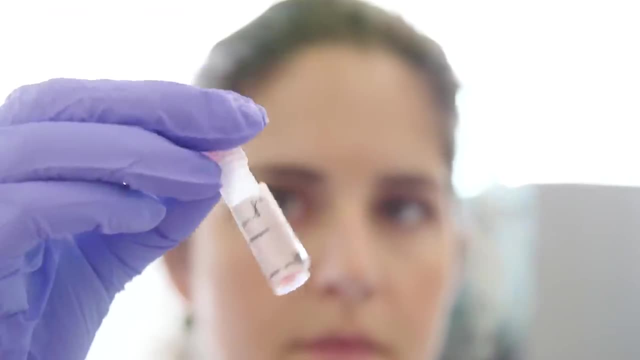 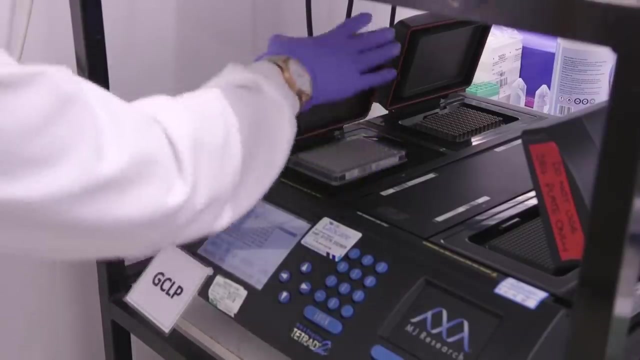 And by comparing genetic information, it's possible to quantitatively measure the relatedness of organisms with data Darwin couldn't have ever dreamed of. With complex algorithms and data analysis aided by massive computing power, the study of evolution and genetics has never been more exciting. 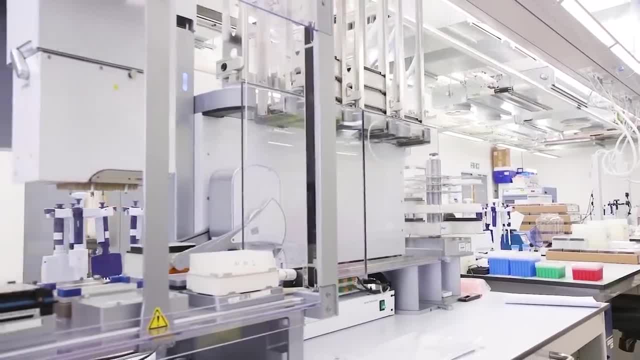 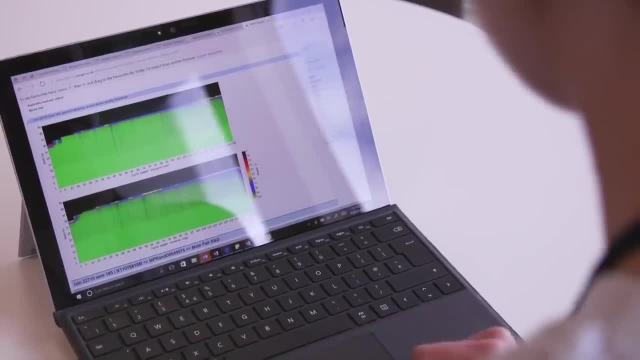 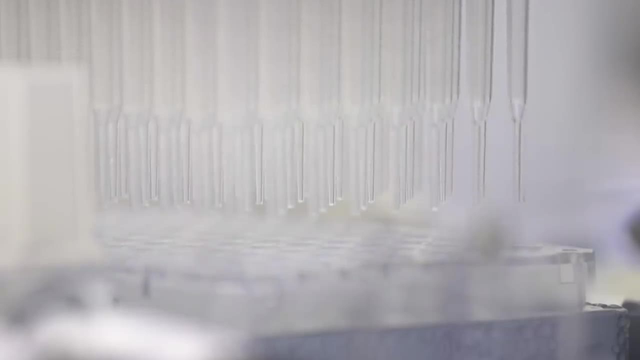 This is the field of computational biology, a field that uses computer science to reconstruct genomes, build phylogenetic trees, to look at evolutionary relationships or unlock the complex folded shapes of proteins. In my opinion, it's the most important field of research happening today, and luckily I've. 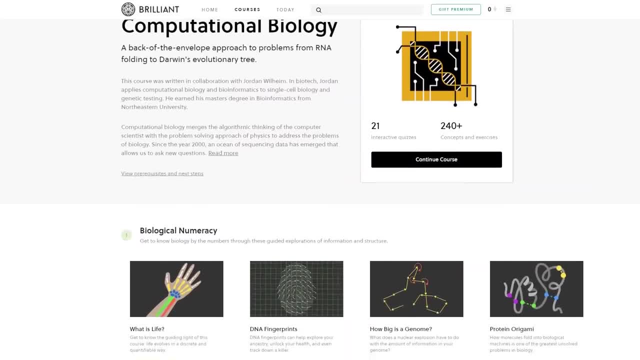 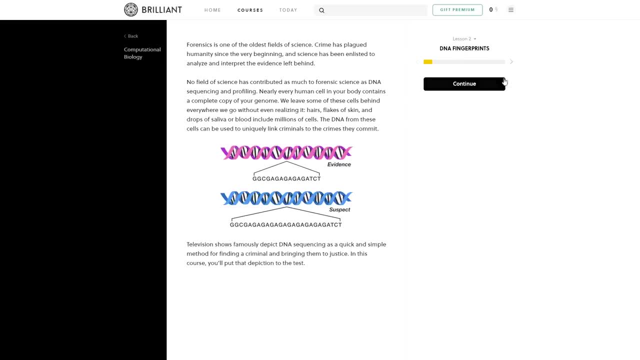 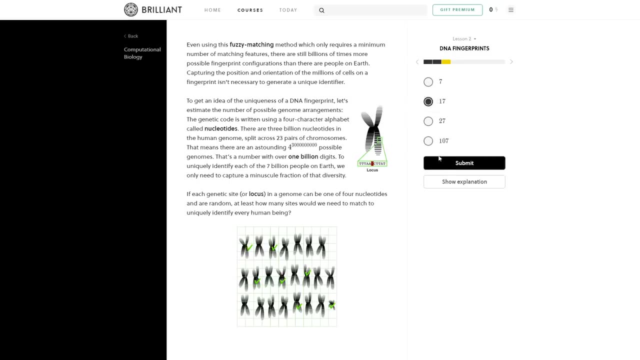 been able to get a solid overview of it from the computational biology course on Brilliant, the online STEM learning platform. It takes what should be a difficult subject and makes it into a fun, colorful and interactive set of lessons and quizzes. It's given me a better understanding of how we know for sure that natural selection 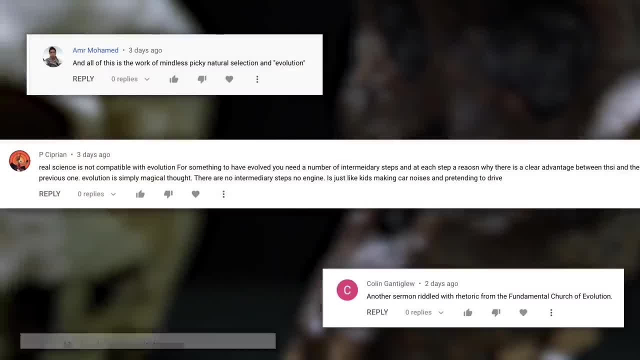 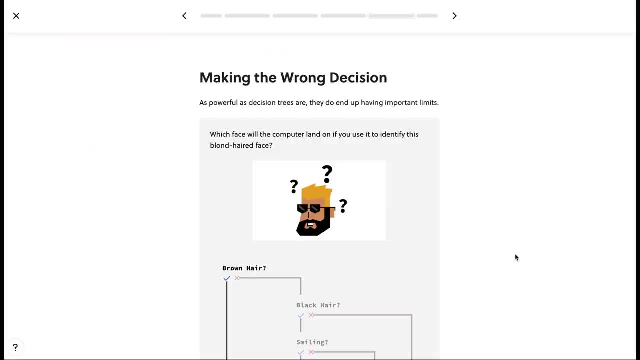 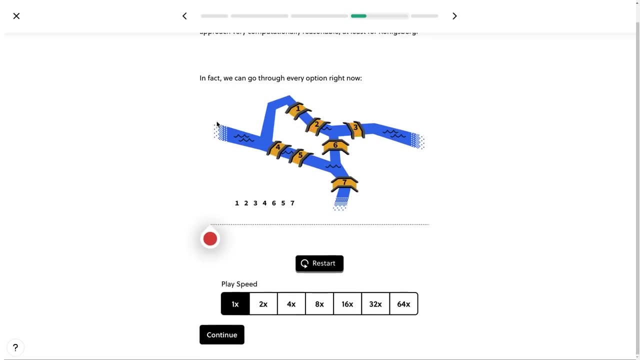 is a provable phenomenon and gives me even more ammunition to argue against the creationists that always seem to flood my comment section. And to take your time To take your learning even further. Brilliant has tons of interactive courses on computer science and math, which, dare I say, are genuinely fun to do. 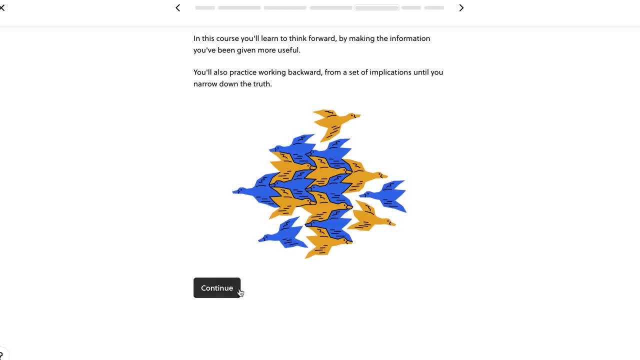 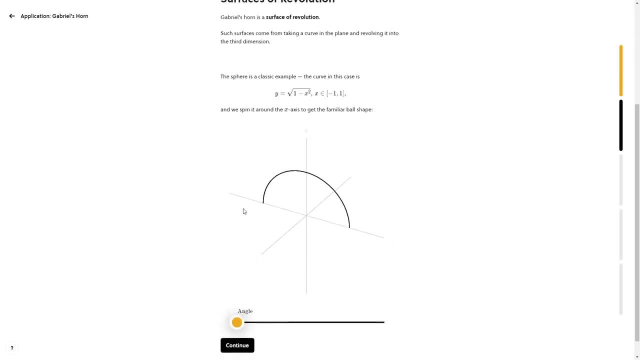 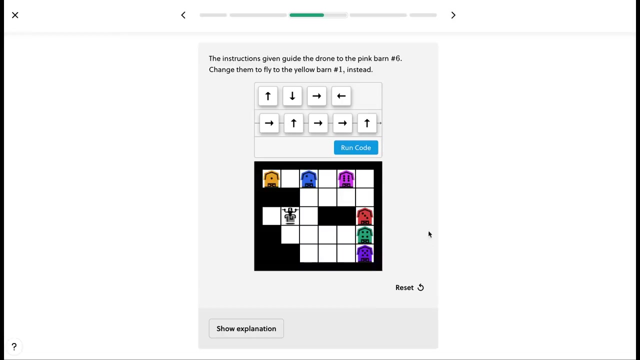 The interactivity makes it easy to learn and is something I wish existed when I was in school. The new year is a great time for building new, healthy habits, and there's no better place to channel that energy than with Brilliant. I've personally been adding a daily computer science fundamentals lesson to my routine. 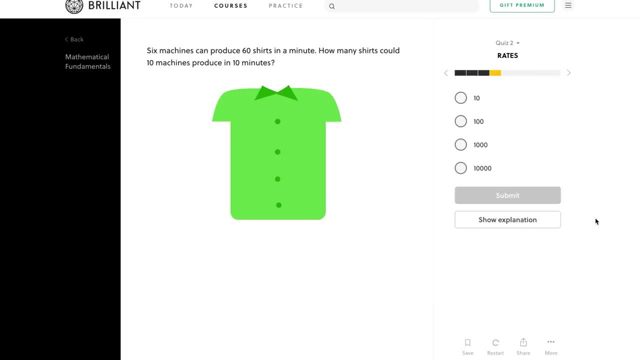 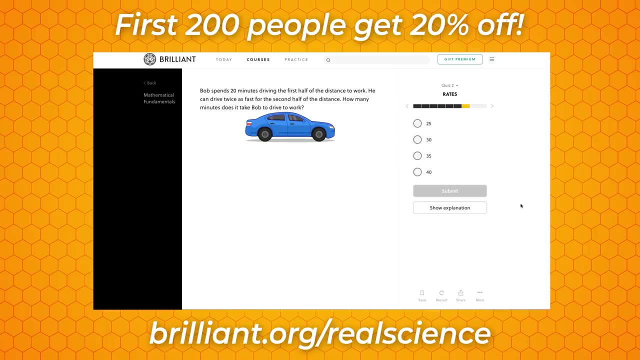 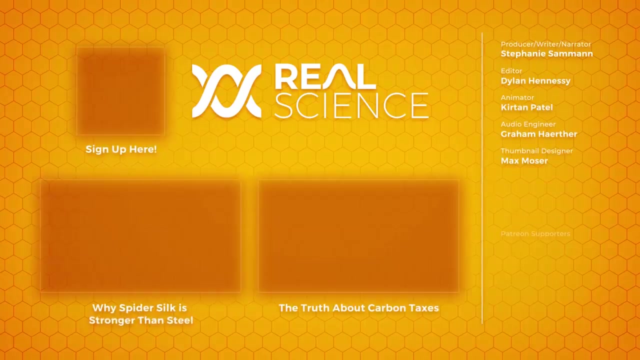 after my daily Wordle. To get started for free, visit brilliant dot org- slash real science, or click on the link in the description and the first 200 people will get 20% off Brilliant's annual premium subscription. As always, thanks for watching and if you're looking for something else to watch, right? 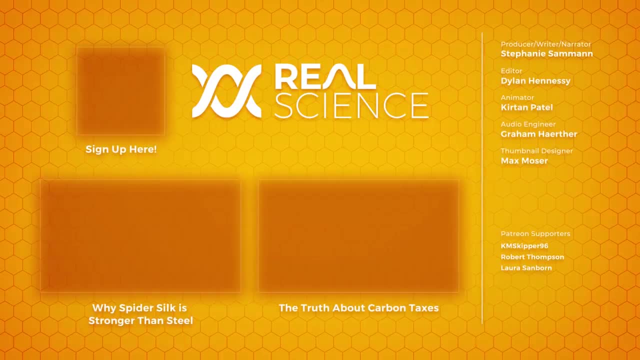 now you can watch our previous video, Why Spider Silk is Stronger than Steel, or Real Engineering's latest video about the reality of carbon taxes. I'll see you in the next one. 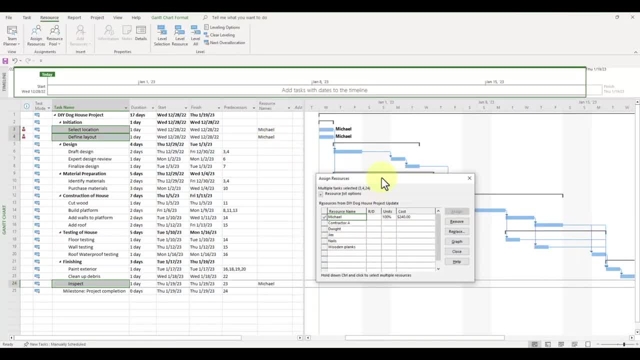 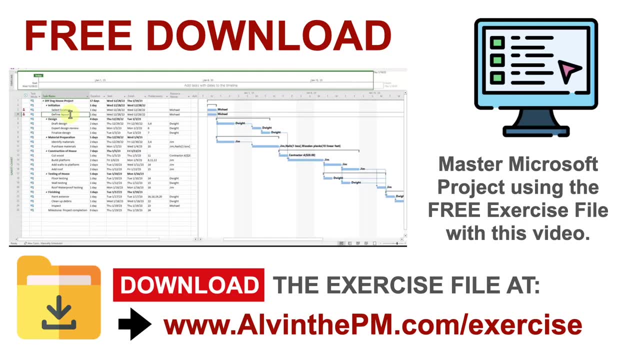 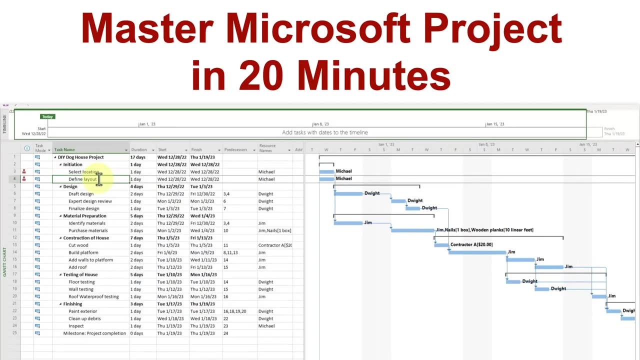 In this video I'm going to teach you how to use Microsoft Project. Download the entire exercise file for free over at alvanthepmcom slash exercise to follow along with this video and learn Microsoft Project the easy way. Alright, so for our example, let's say you're working on a very simple DIY project to build. 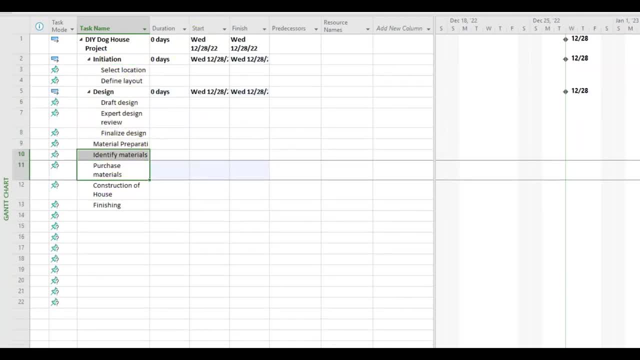 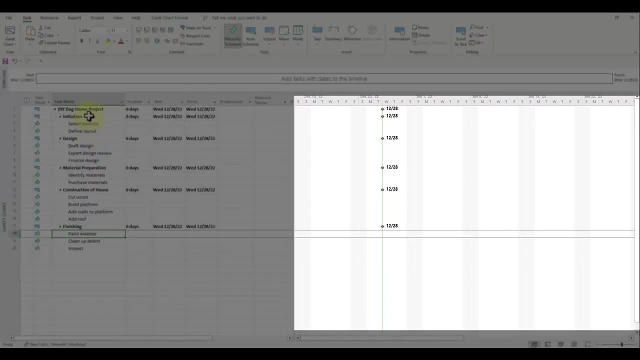 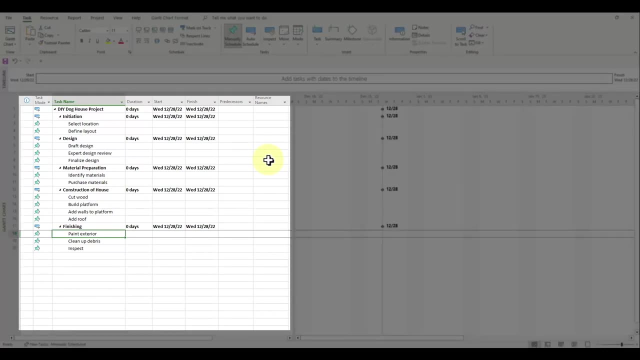 your own doghouse and you want to create a schedule and a total cost estimate using Microsoft Project. Microsoft Project's interface is split up into two areas. The right side is the Gantt chart view, which graphically shows your project schedule using bars, And the left hand